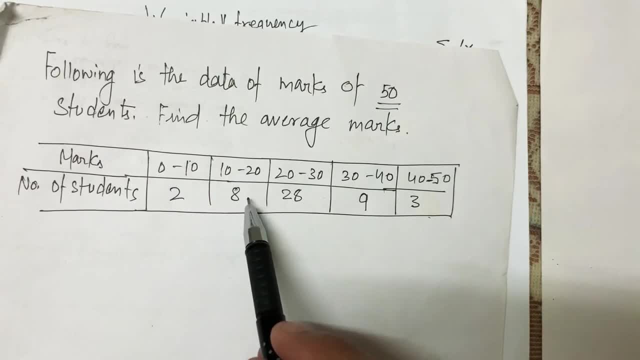 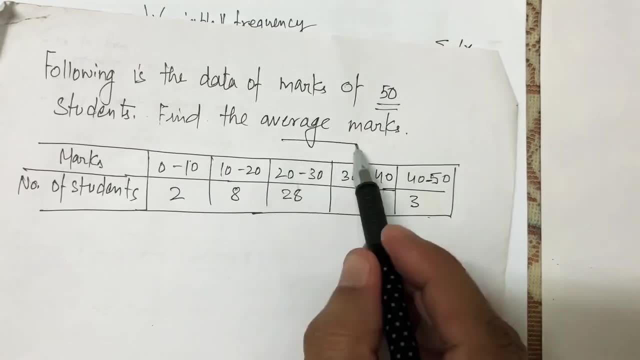 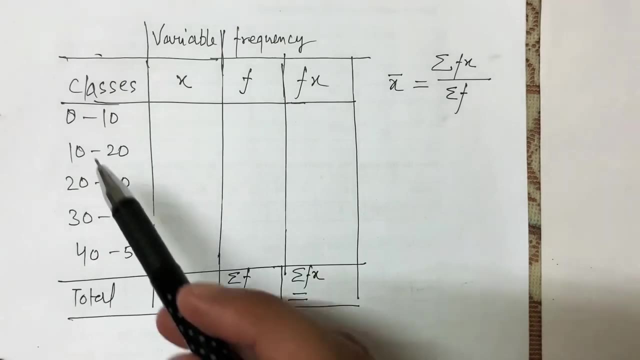 somebody is scoring exactly 10 marks, the student is going to fall into the next class. That means upper limit of each class is excluded and my objective is to find out average marks. So this is where I have written the question in a tabular format. So I have classes of marks you can see 0. 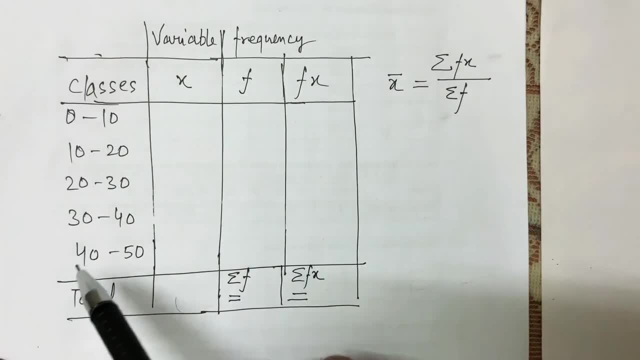 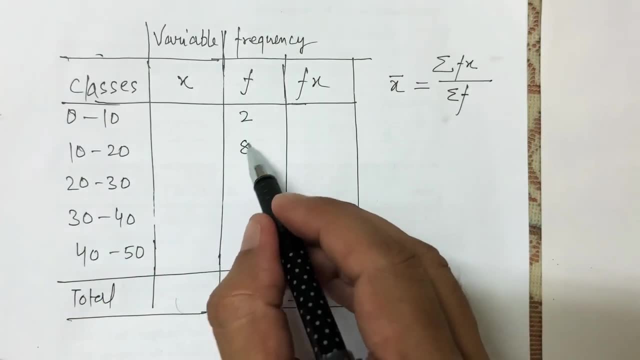 to 10,, 10 to 20,, 20 to 30,, 30 to 40,, 40 to 50 and I have been given in the question with the frequency, which is there are two students who are scoring between 0 to 10,. there are 8 students who are scoring between 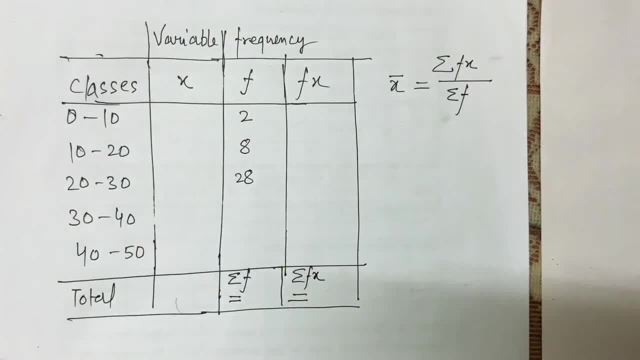 10 to 20, there are 28 students scoring between 20 to 30, and 30 to 40, there are 9 students, and 40 to 50 there are 3 students, and this gives me a total of 50 students. So in total, there are 50 students. 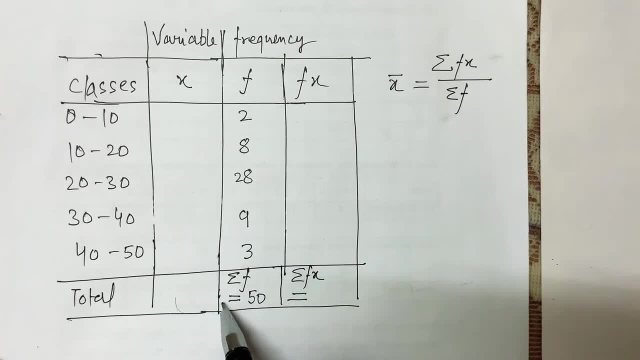 in the class. and that is all the summation of F, or I can also represent it by the letter capital N, which is the total number of observations in the data set, and I want to find out the average marks. that means the X bar. Now here I know the. 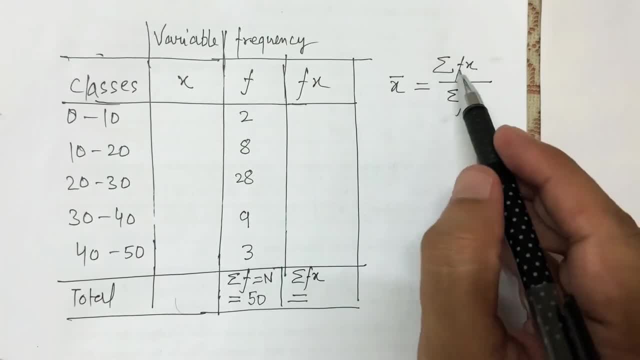 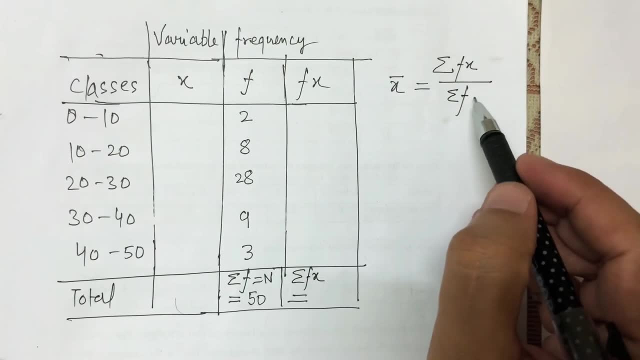 formula of X bar is summation of Fx divided by sum of F. Summation of Fx gives me the sum of total marks scored by all the students and sum of F gives me the total number of students in the class which I have already calculated they are in. they are 15 numbers. So in order to get summation Fx, I 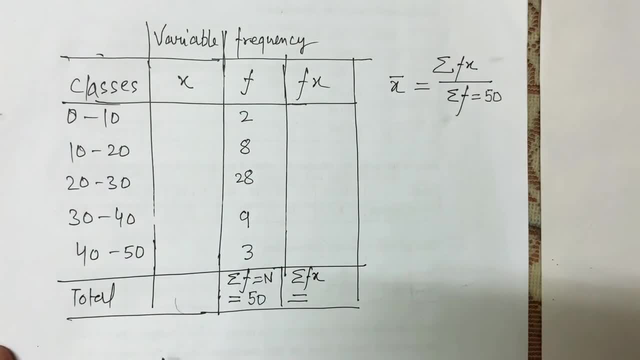 do not have a direct value of x here. I have been given with the continuous classes, so I obtain the value of x, And then I have theario value and the cap value from the class which is also called as mid value. This is also called as the mid value, and the middle value can be obtained by upper limit plus lower. 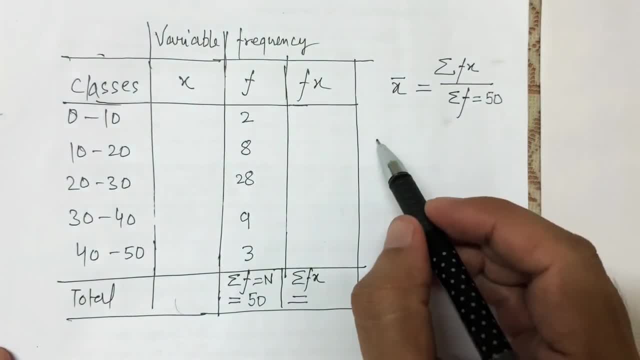 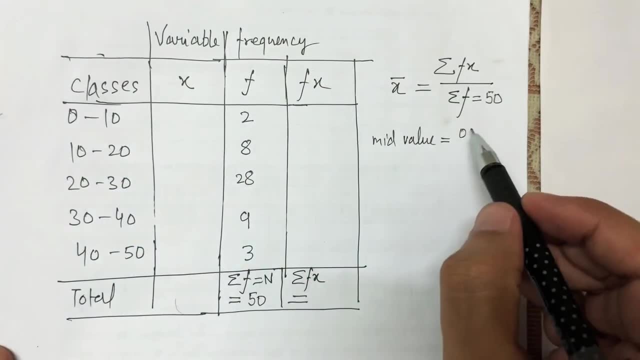 limit of any class divided by 2.. So the mid value- I am going to just make a calculation here- for first class- mid value for first class is going to be 0. that means the lower limit plus the upper limit, that is 10, of this particular class divided by 2.. 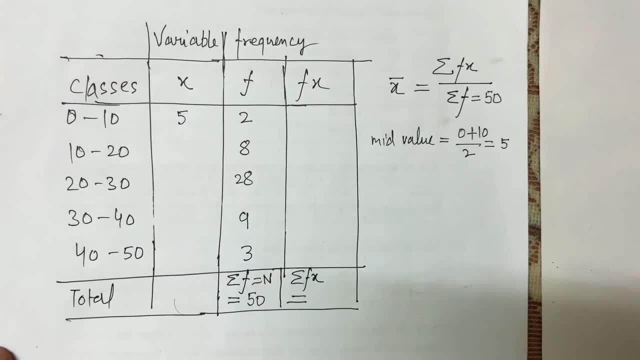 And that gives me a value 5.. value for this class is 5. now, same way, I am going to calculate the mid value for rest of the classes. for this it will be 10 plus 20 divided by 2. that is going to give me the.